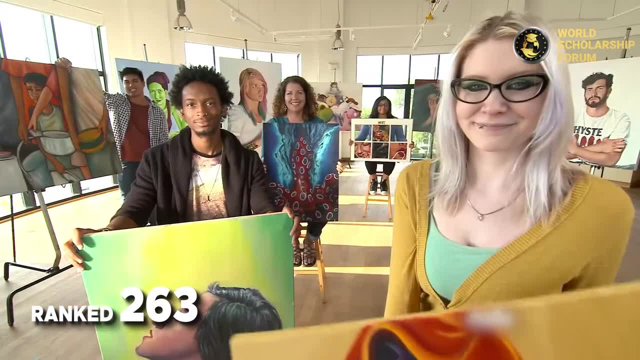 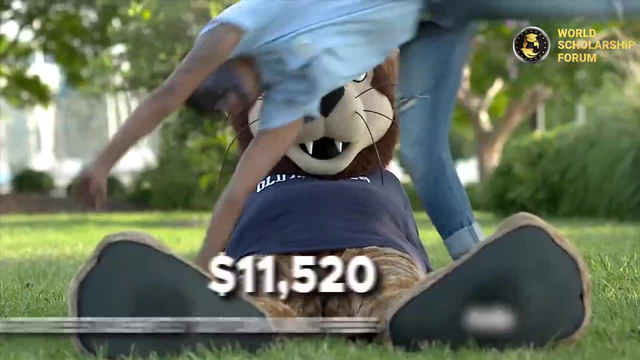 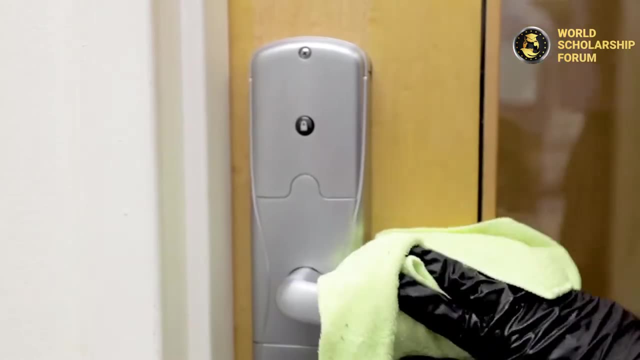 Old Dominion University is ranked number 267.. an International International University called Old Dominion University for 1863 in National Universities. It charges $11,520 for In-State tuition and fees and $31,680 for out-of-State tuition and fees. The Old Dominion University, which was originally 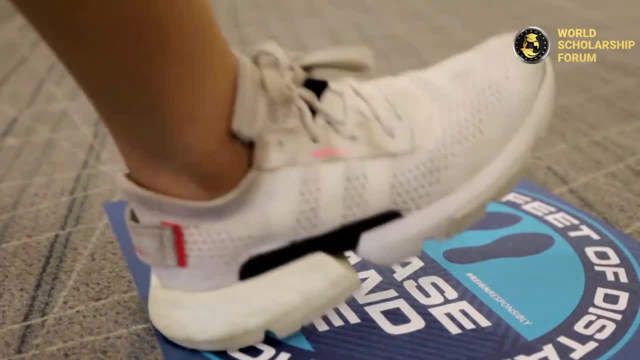 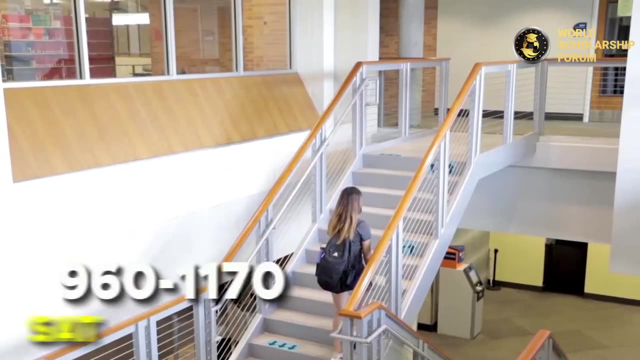 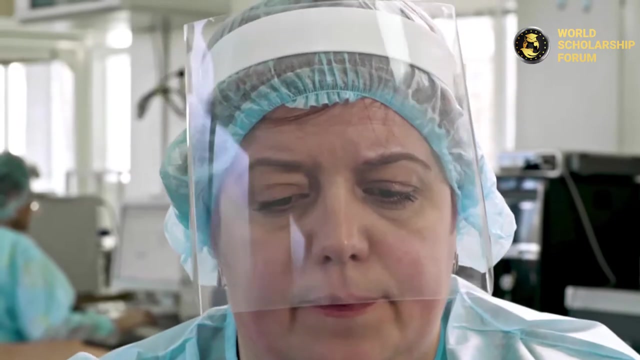 a branch of William & Mary, is now a standalone university in Norfolk, Virginia. Admission to Old Dominion University is competitive with a 95 percent acceptance rate. 70 or an ACT score of 18 to 25 is required for admission to Old Dominion. Old Dominion. 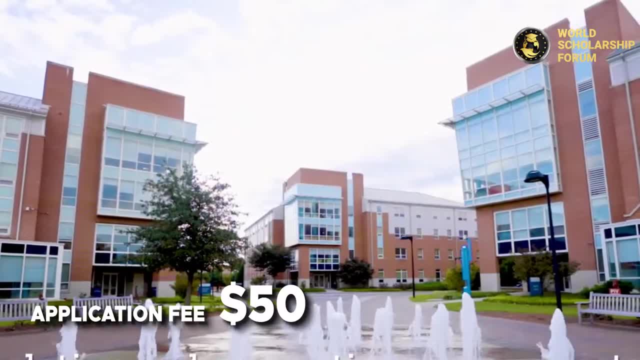 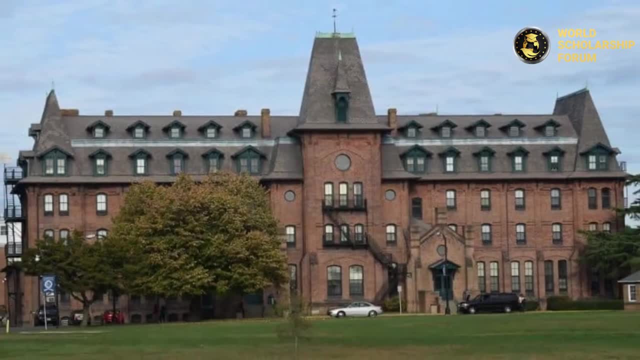 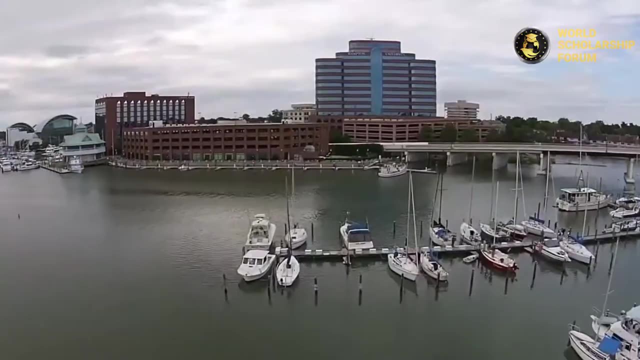 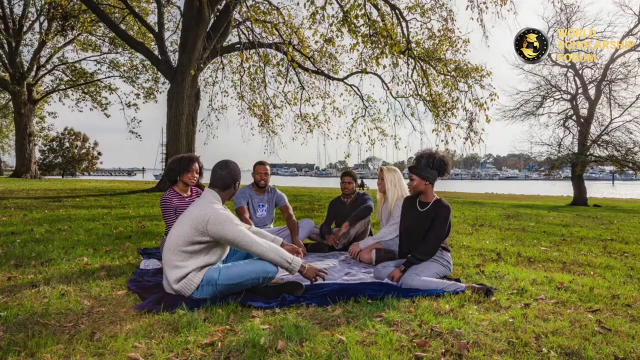 University charges a $50 application fee. Number 2. Hampton University. Hampton University is sixth of the best colleges in Virginia. Hampton University was established in 1868 as a private institution. It is located in an urban area and covers 314 acres. The academic calendar is: 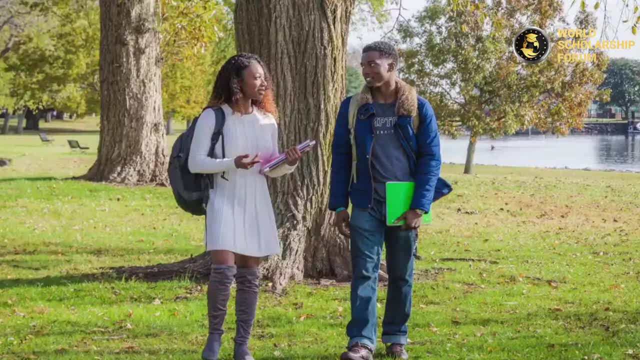 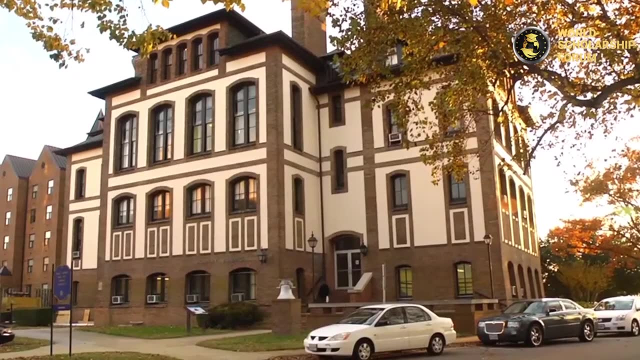 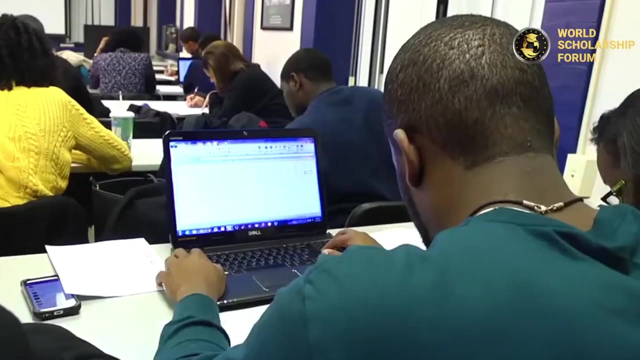 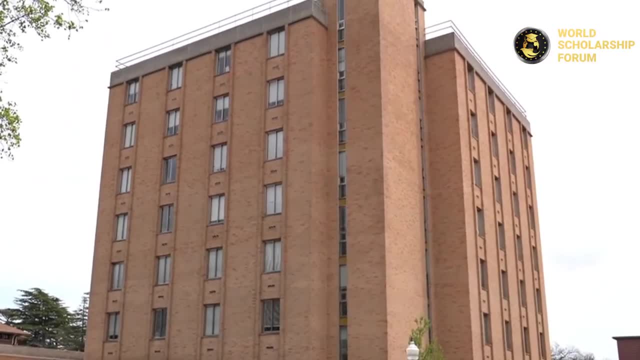 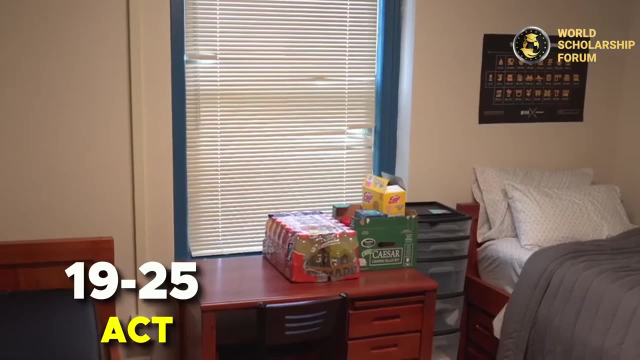 The university's admissions process is competitive, with just 36% of applicants being accepted with a $49,287 fee. Half of Hampton University's admitted students had an SAT score of 980 to 1160 or an ACT score of 19 to 25.. 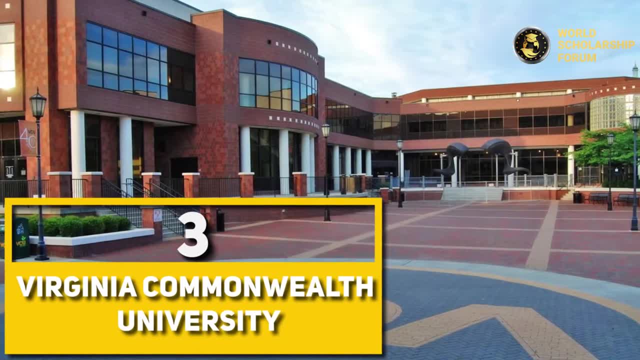 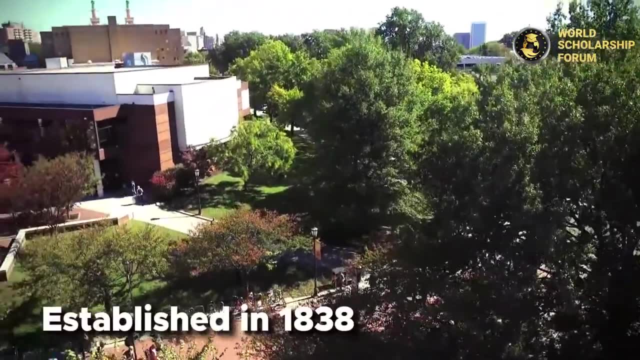 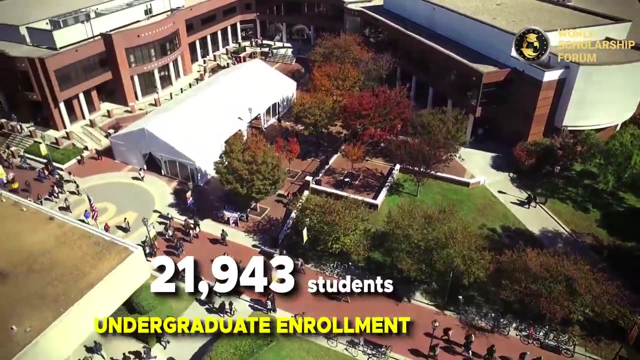 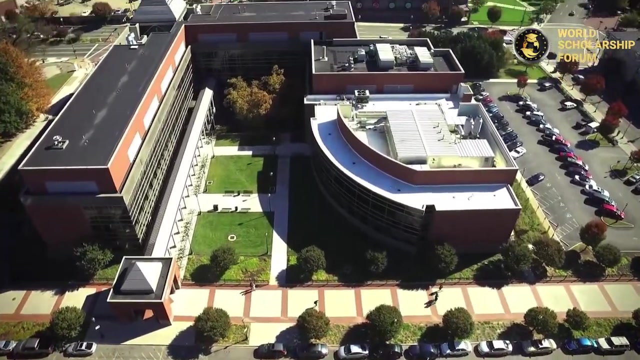 Number 3. Virginia Commonwealth University. Virginia Commonwealth University is the fifth best college in Virginia and was established in 1838 as a public university. It has a total undergraduate enrollment of 21,943 students. fall 2020 is located in an urban area and covers 168 acres. the academic calendar is semester based. in the 2022 edition of best colleges, virginia commonwealth university is ranked number 172 in national universities. in-state students tuition and fees are fifteen thousand and twenty eight dollars, while out-of-state tuition fees are thirty five thousand six hundred and seventy six dollars. 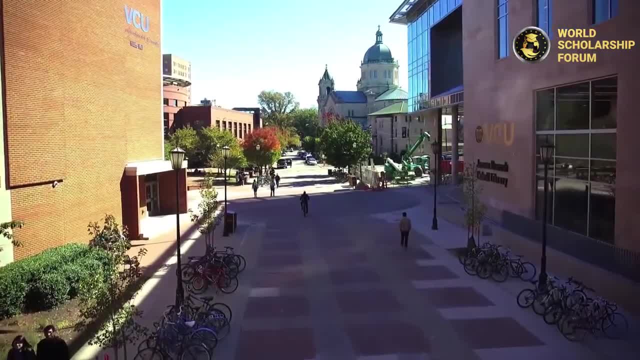 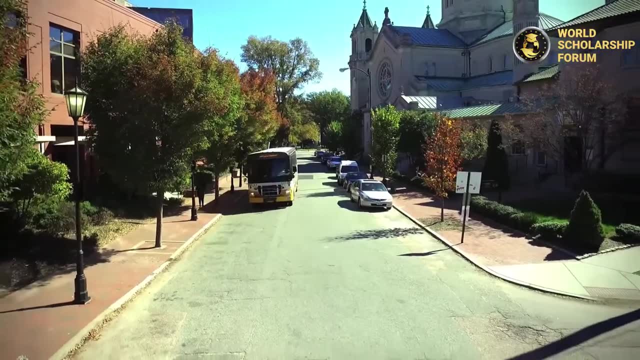 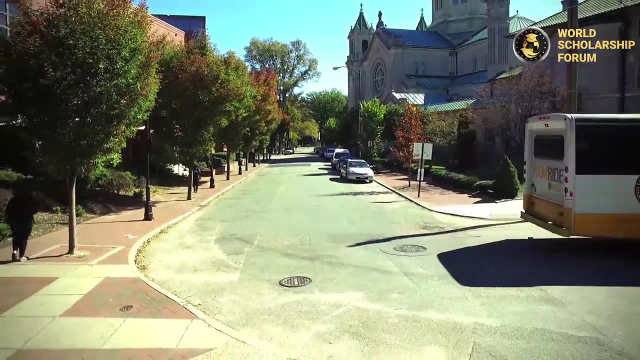 admission at virginia commonwealth university is competitive with a 91 acceptance rate. it admits half of its candidates with an sat score of 1060 to 1250 or an act score of 21 to 28.. virginia commonwealth university charges a 70 application fee. 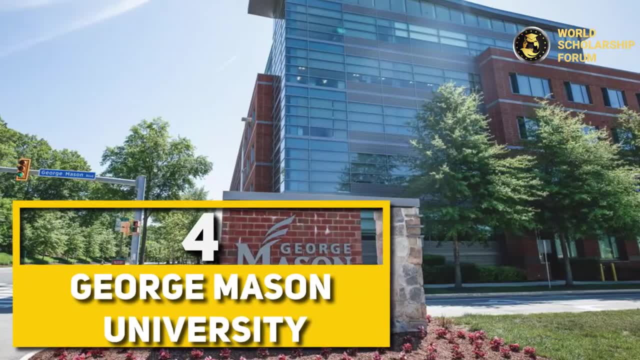 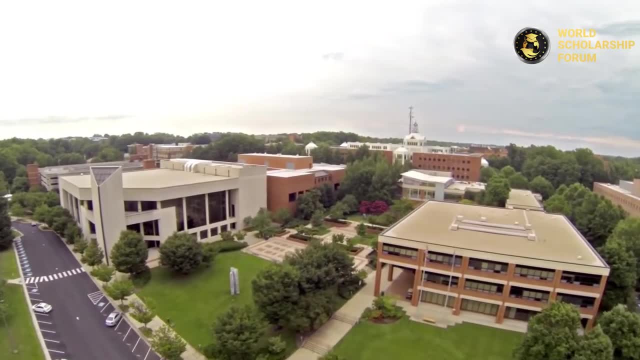 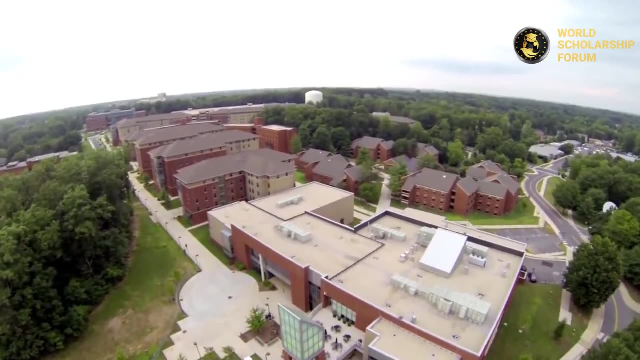 number four: george mason university. george mason university opened its doors in 1972. george mason university has three suburban campuses in northern virginia and an international campus in sondo, korea, near columbia. in the 2022 edition of best colleges, george mason university. is ranked number 148 in national universities. in-state students tuition and fees are thirteen thousand one hundred and nineteen dollars, while tuition and fees for out-of-state students are thirty six thousand five hundred and seventy nine dollars. admissions at george mason university is competitive, with an acceptance rate of eighty nine percent and a ninety percent early acceptance. 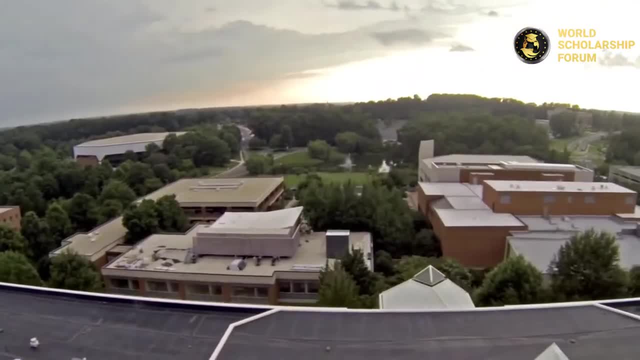 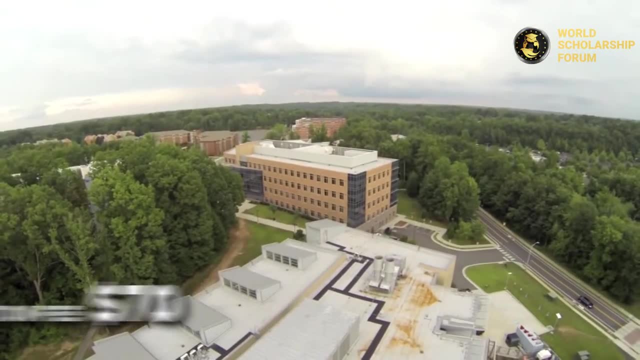 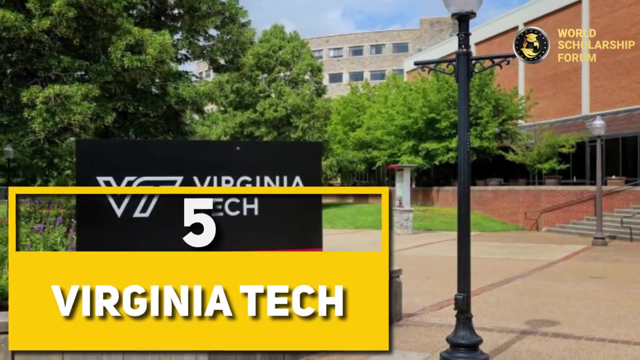 rate, half of the admitted students have an sat score of eleven hundred to thirteen hundred or an act score of twenty four to thirty. george mason university charges a seventy dollar application fee. number five: virginia tech. virginia tech was established in 1872 as a public university. 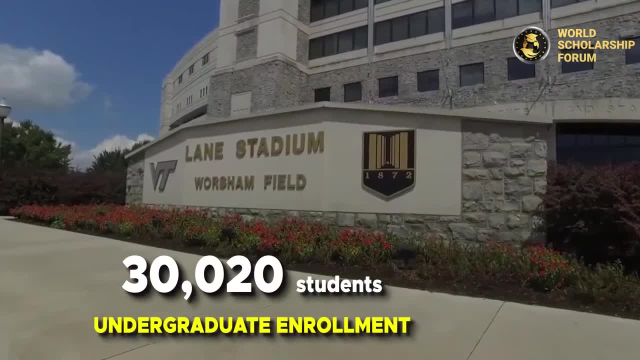 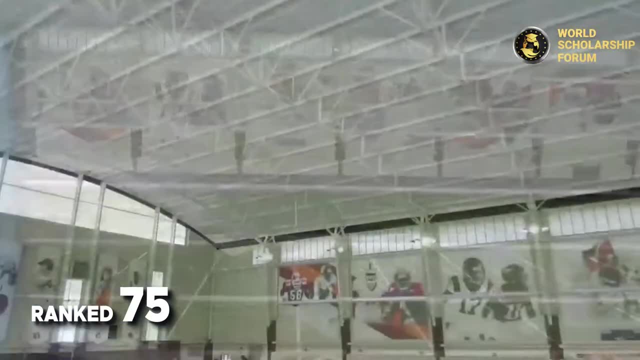 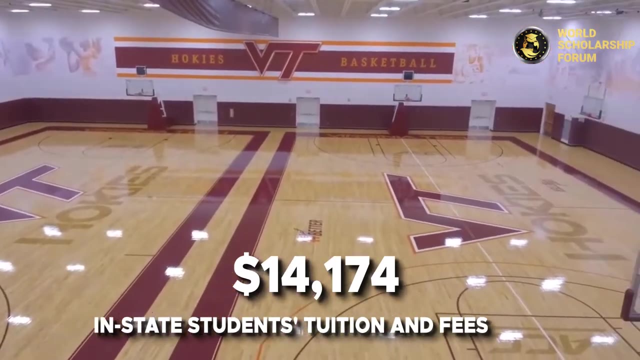 it has a total undergraduate enrollment of thirty thousand and twenty students on a two thousand six hundred acre campus. virginia tech has ranked number 75 in national universities in the best colleges 2022 edition. it charges fourteen thousand one hundred and seventy four dollars for in-state tuition and 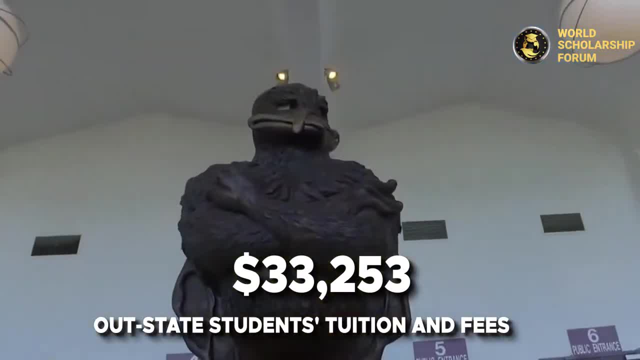 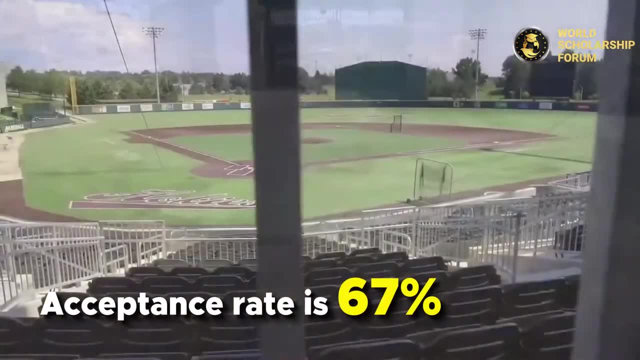 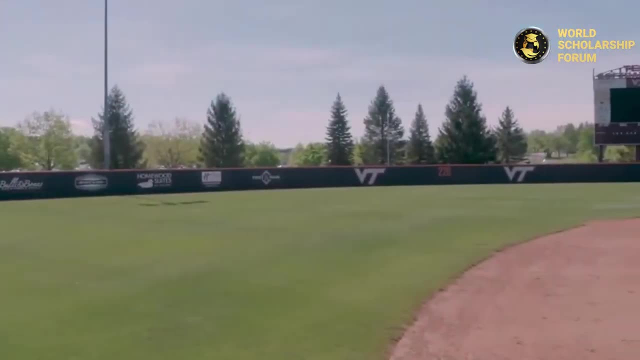 fees and thirty three thousand two hundred and fifty three dollars for out-of-state tuition and fees. virginia tech admissions are more selective, with a 67 percent acceptance rate and a 77.3 percent acceptance rate, as well as a 65 graduation rate. half of the admitted students had an sat. 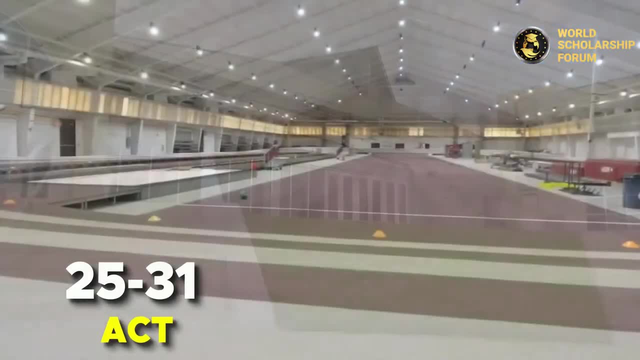 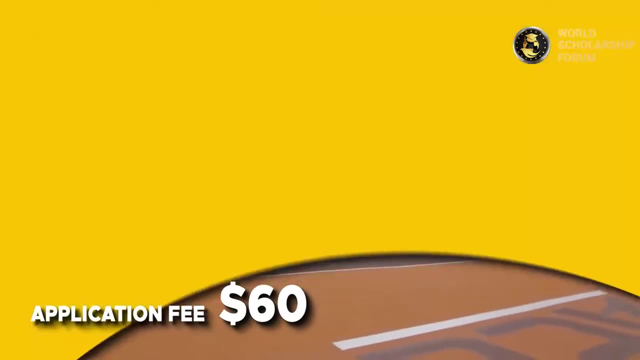 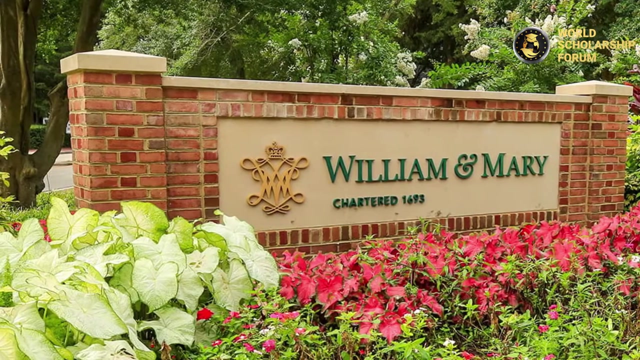 score of 1170 to 1370 or an act score of 25 to 31.. virginia tech charges a 60 application fee. number six: william and mary. william and mary are one of the best colleges in virginia that were established in 1693.. william and mary in williamsburg, virginia, is the country's 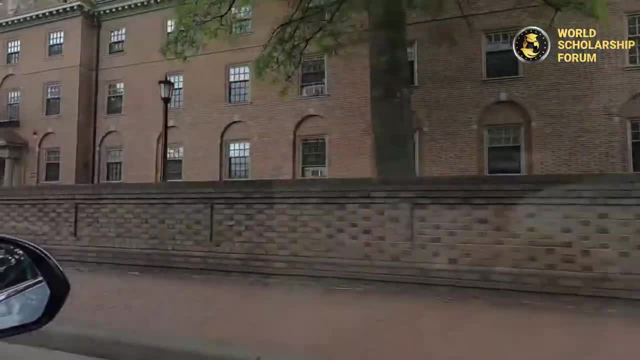 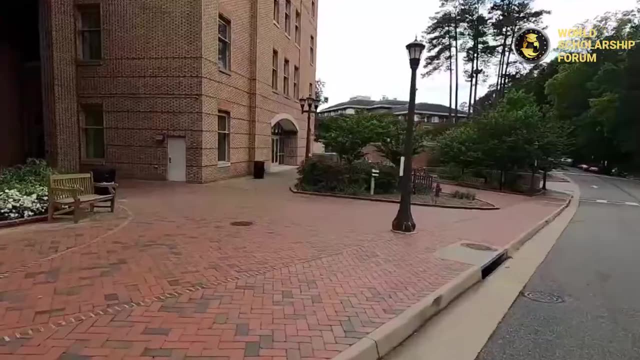 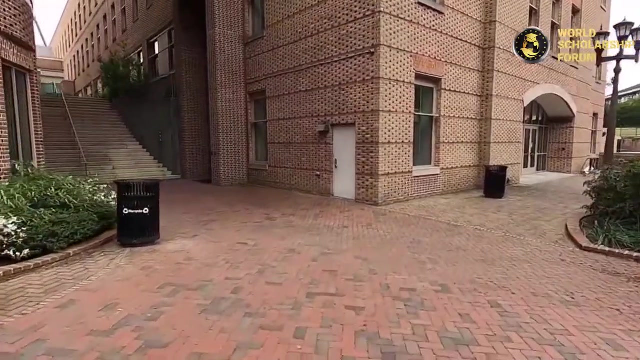 second oldest college. the institution was created in 1693 by king william iii and queen mary ii of england. admissions at william and mary is highly selective, with a 42 acceptance rate and an 85 graduation rate. half of william and mary's admitted students have an sat score of 1300. 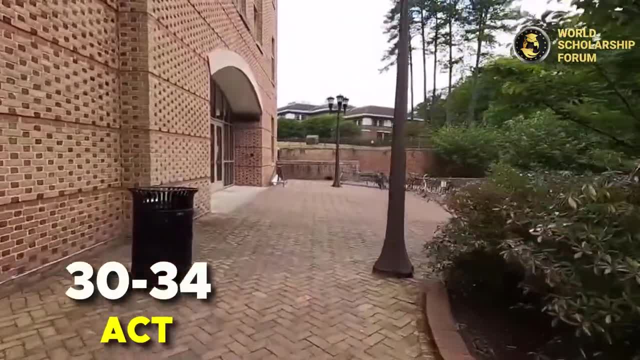 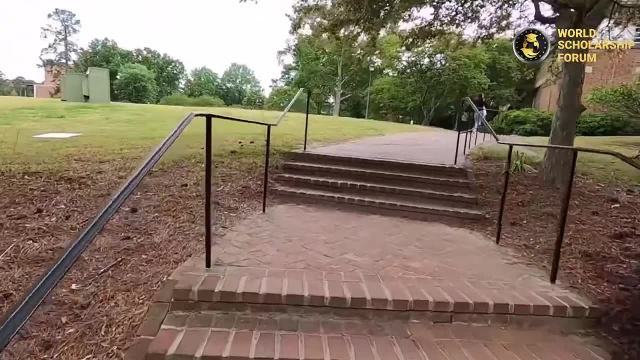 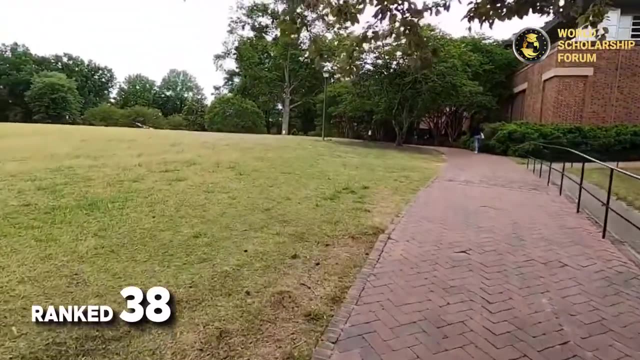 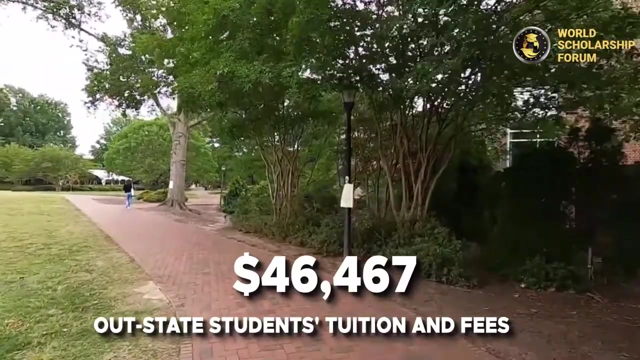 to 1490, or an act score of 30 to 34.. william and mary charges a 75 application fee. in the 2022 edition of best colleges, william and mary is ranked number 38 in national universities. tuition and costs for in-state students is 23 812, while out-of-state students pay 46 467. 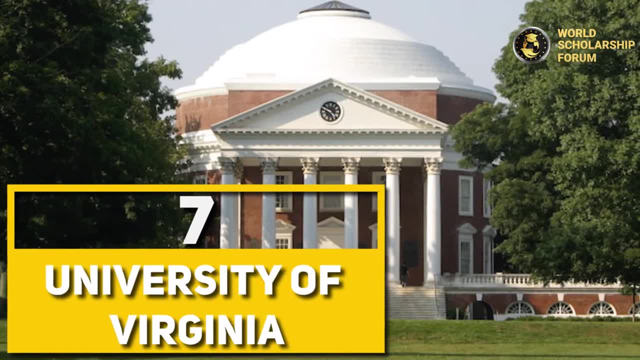 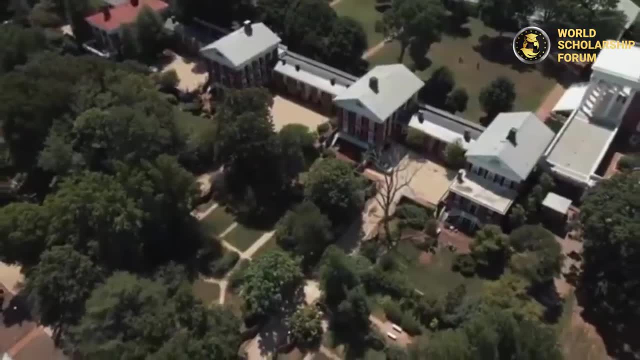 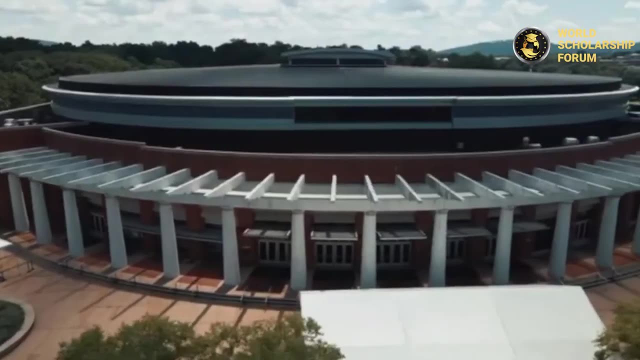 number seven: university of virginia. the university of virginia is the best college in virginia, founded by thomas jefferson in 1819.. charlottesville is home to the university of virginia. only first-year students must reside on campus, while many upper-level 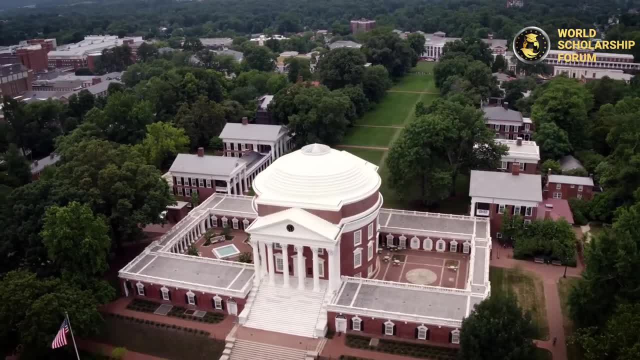 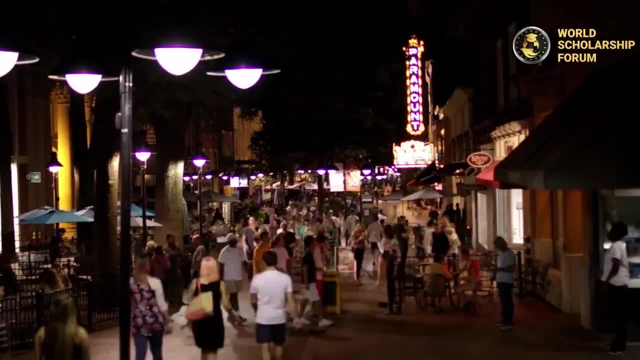 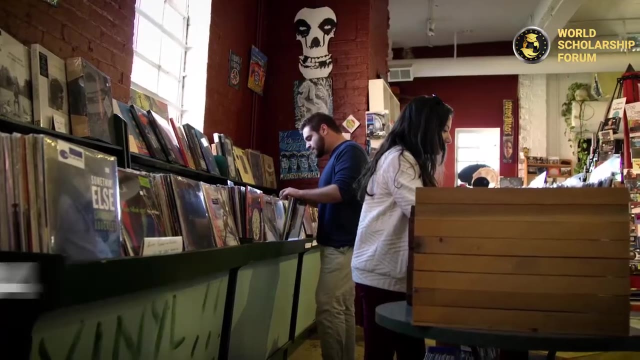 students live off campus. university of virginia admissions is the most selective, with a 23 acceptance rate and a 20.6 early acceptance rate. an sat score of 13, 20 to 15, 10 or an act score of 30 to 34 is required for admission into the university. the university of virginia has ranked 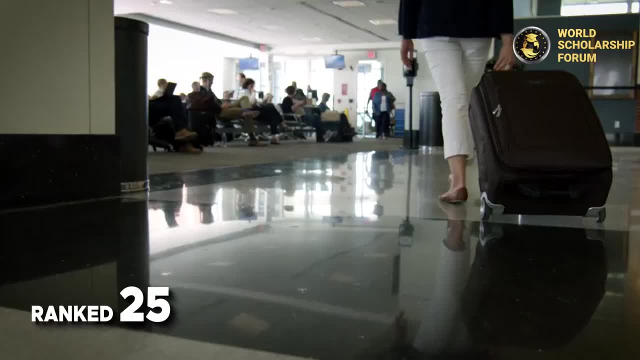 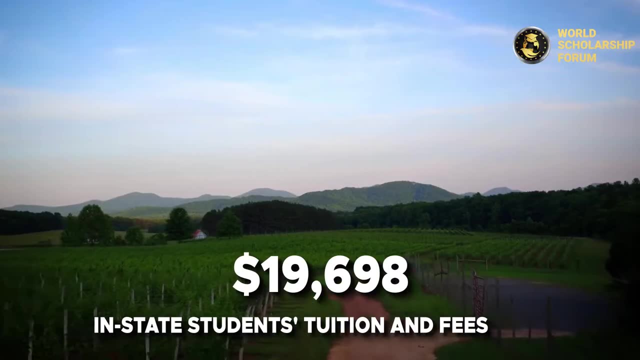 number 25 in national universities. university of virginia has ranked number 25 in national universities universities in the best colleges 2022 edition and number one in virginia. it charges nineteen thousand six hundred and ninety eight dollars for in-state tuition and fees, and fifty three thousand. 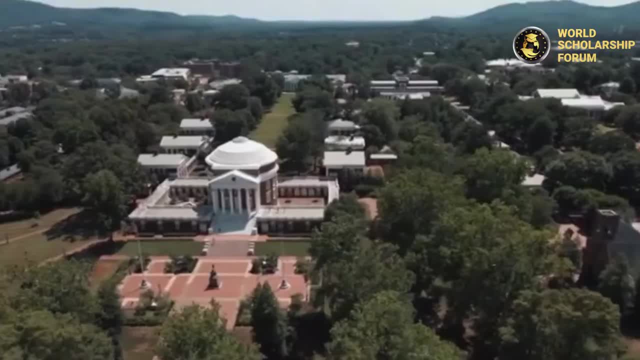 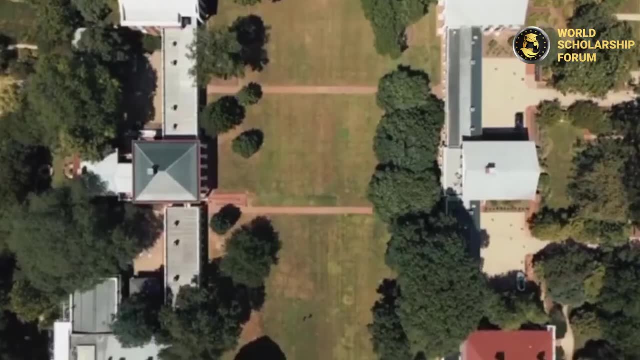 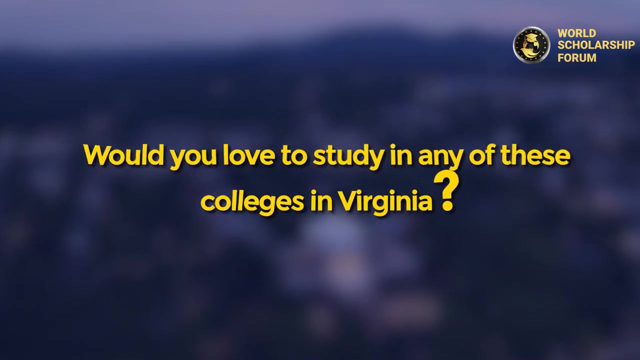 six hundred and sixty six dollars for out-of-state tuition and fees. virginia has risen to the top of cnbc's america's best states list for business. this rating was influenced by the state's highly skilled and educated workforce. would you love to study in any of these colleges in virginia? 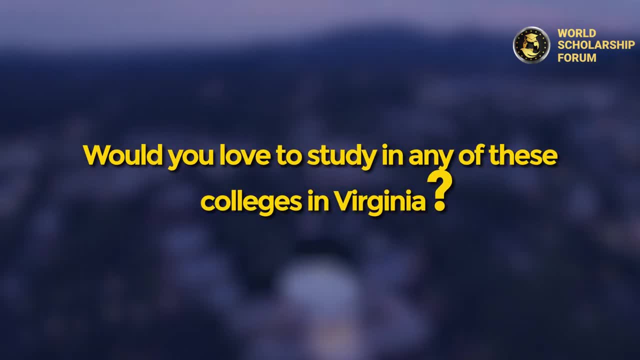 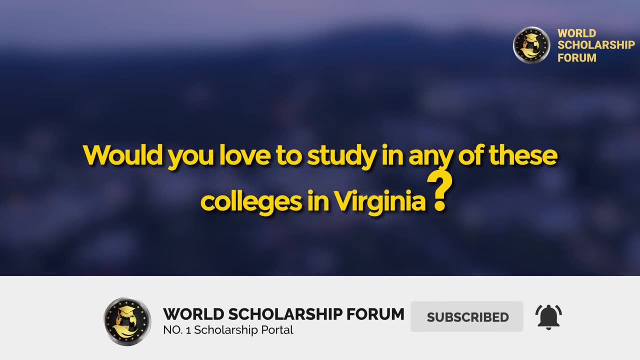 virginia. let us know in the comments section below. thanks for watching. don't forget to click the subscribe button and ring the notification bell to be the first to watch new videos on this channel.